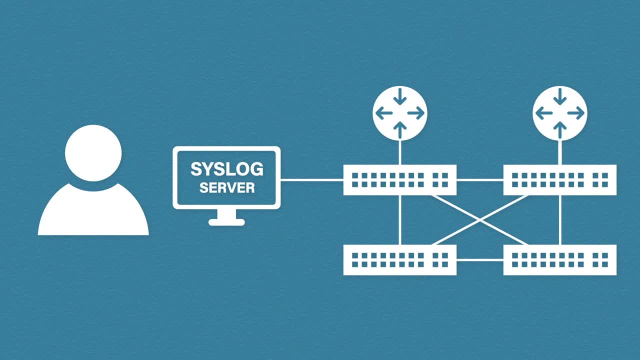 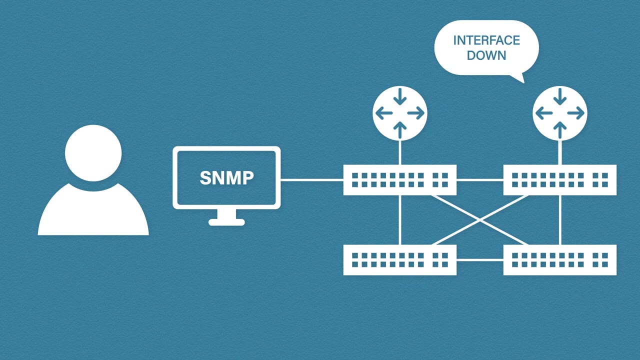 that can help make network monitoring easy. He then discovered SNMP. Using SNMP, Bill can now actively monitor the health of his network, all from the comfort of his own chair. If an interface goes down on one of his routers, he's quickly alerted to the change and he can leap into action. 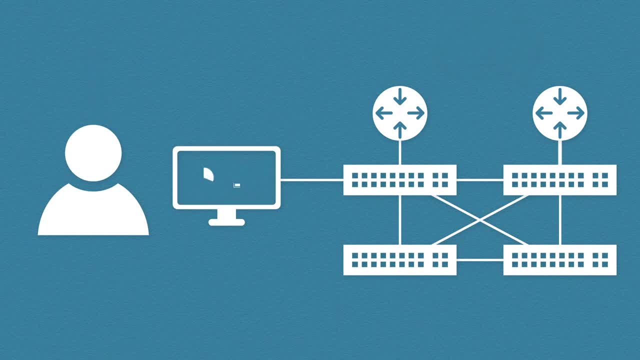 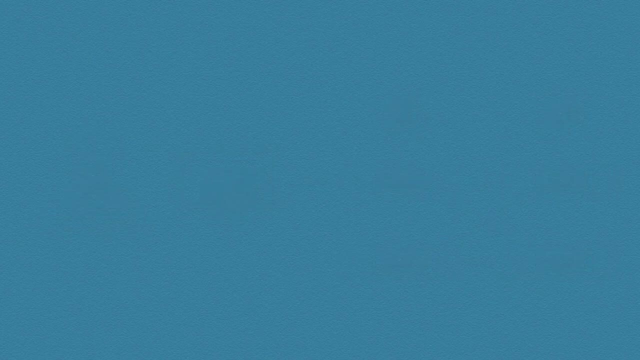 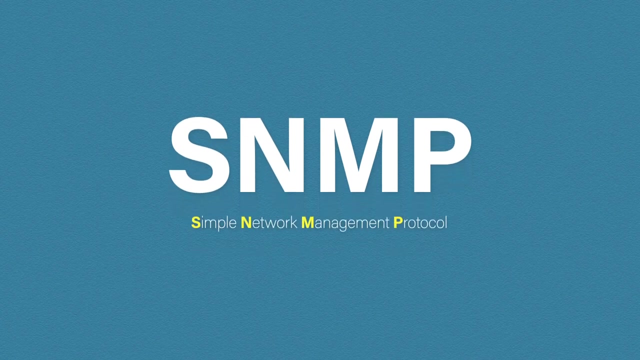 And it doesn't stop there. He can monitor the network bandwidth, CPU usage and even the temperature of his devices. This is all possible with the SNMP protocol. So let's take a step back. What is SNMP? SNMP stands for Simple Network Management Protocol. It's a standardized 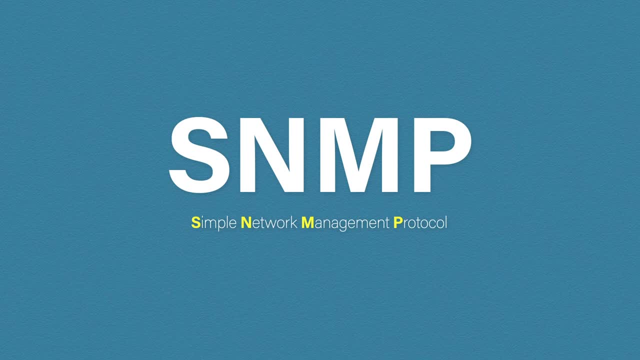 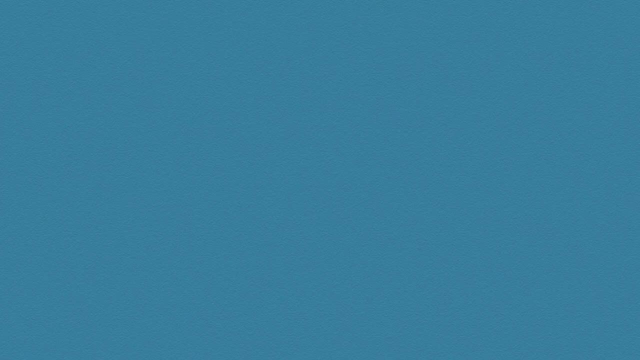 protocol used to collect and organize device information on the network. It's a standardised protocol used to collect and organise device information on a network. It does this over UDP port 161.. Okay, so to see how this works, let's take this. 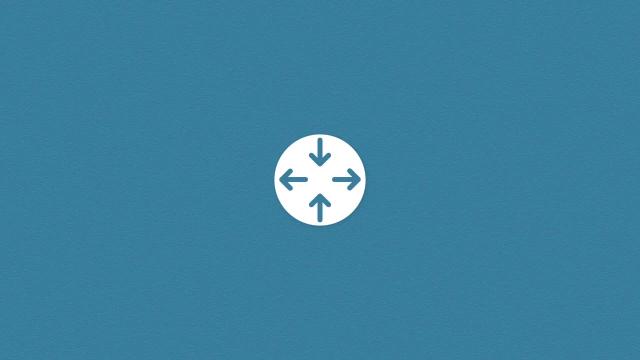 router as an example. A device that is SNMP enabled is known as an agent. An agent has several objects that can be interacted with. Some objects are part of an industry standard and some will be vendor specific for this device, For example, this router will have objects for. 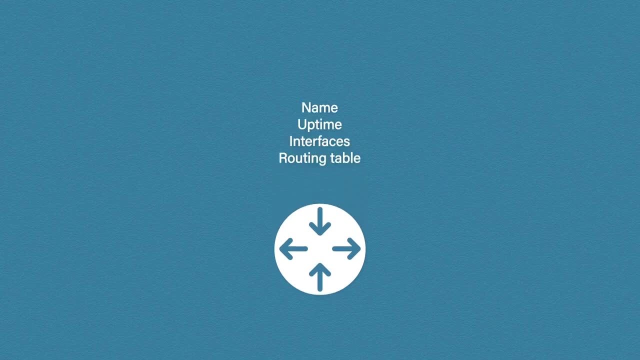 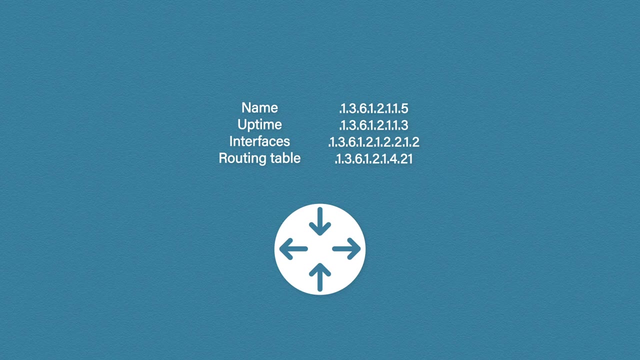 the name, the uptime, the interfaces and the routing table, to name just a few. Each object is assigned a object identifier or OID. The OID is a sequence of numbers which at first glance can look like an IP address. This is used to identify the object. These OIDs are stored in a file called a MIB. 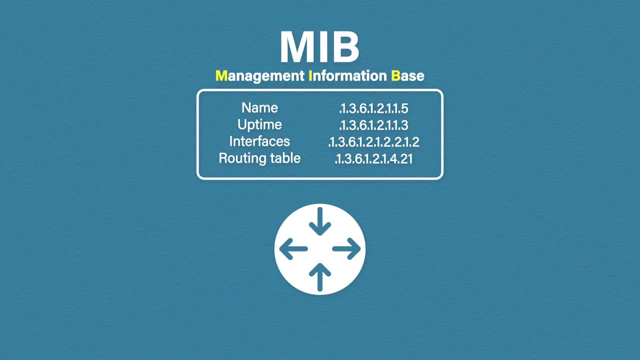 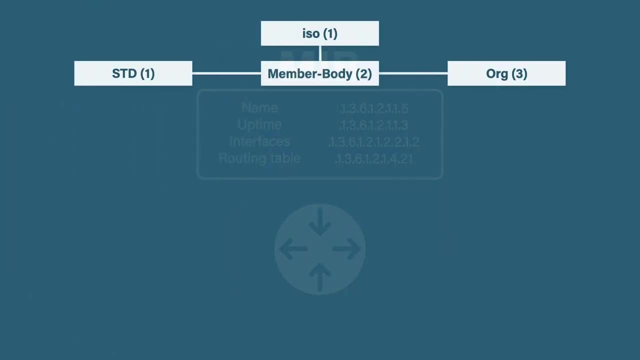 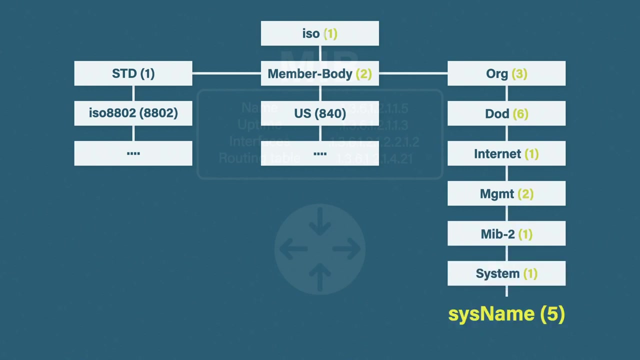 which stands for Management Information Base. The MIB itself follows a tree structure. This is an example of the MIB structure for this sys name object. As you can see, each level has a number. This is where the OID number comes from. It tells the. 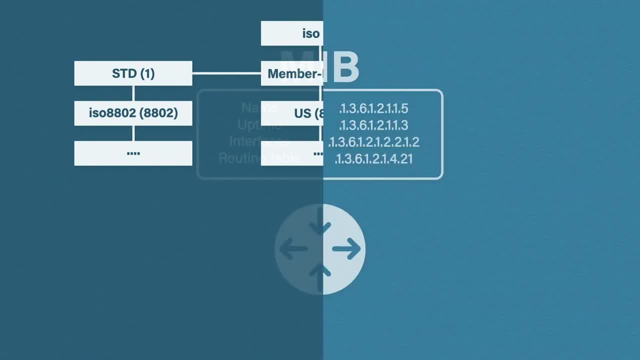 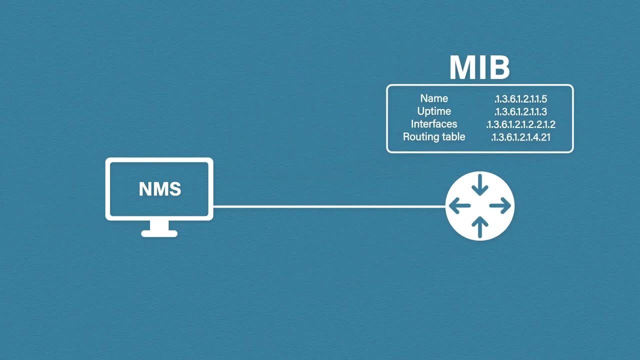 agent, the exact location of the object. So that's the agent and the MIB. But to interact with these objects we need something called a Network Management System, or NMS. The NMS is a piece of software that can be used to take data from the NMS and the system in particular. This is a 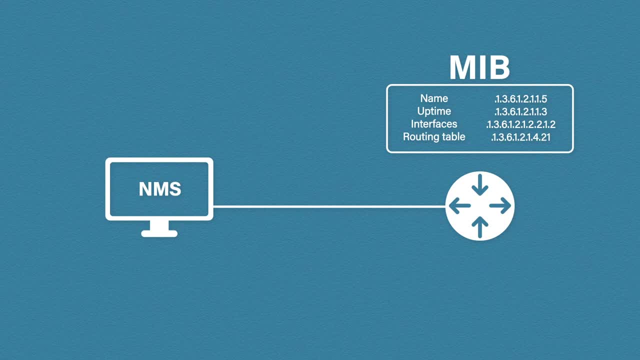 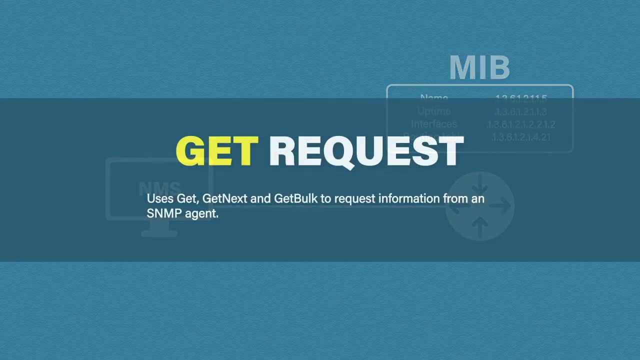 communicate with the SNMP agent. There are a few ways the NMS can speak to the agent. The first way is by using GET requests. GET messages include GET, GET-NEXT and GET-BULK. They are used to actively request information from the agent. For example, our NMS may ask: 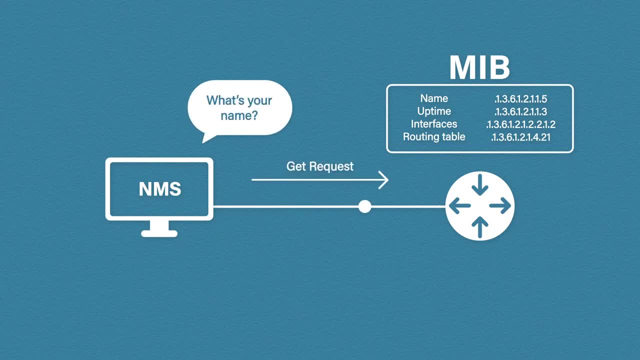 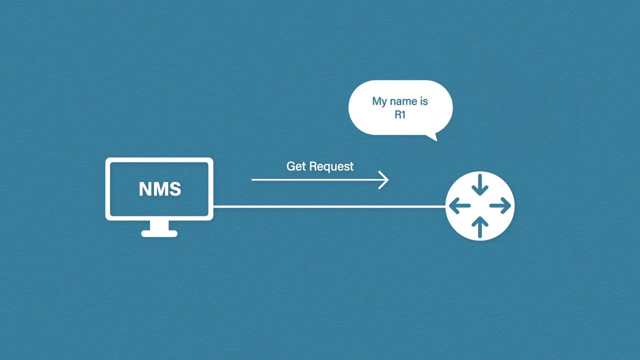 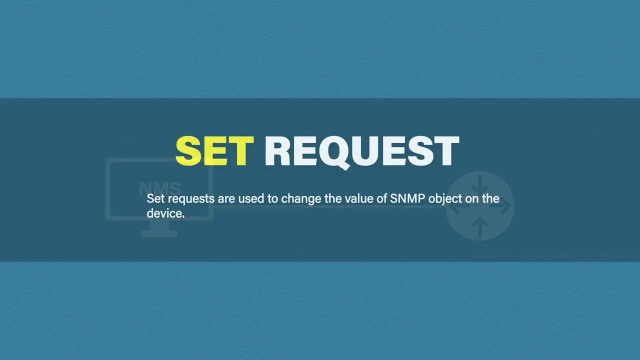 what is your name and it sends a GET request. The agent will then see this request for the name object and it replies with: my name is R1 and it sends a GET response back to the NMS. The second way we can talk to an agent is by using SET requests. The SET request is used to change. 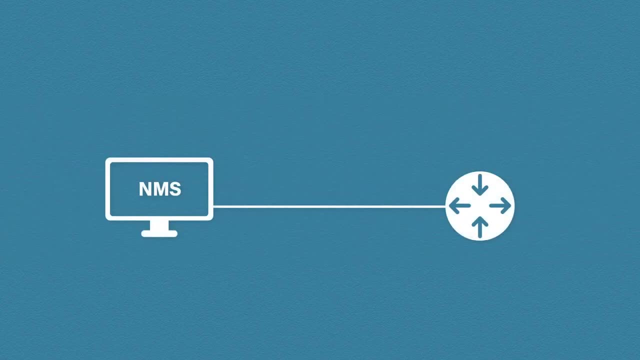 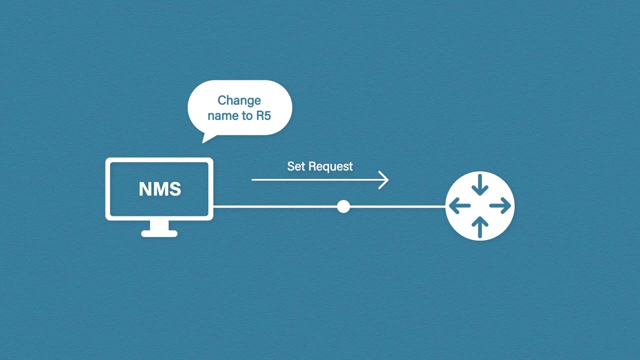 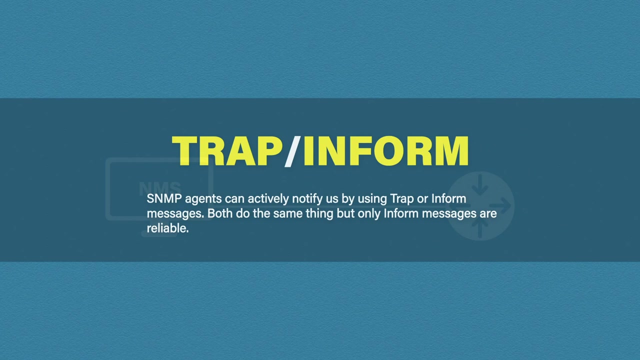 the value of an object on the agent. For example, our NMS might say: change your name to R5 and it sends a SET request. The agent changes this name to R5 and sends a response back. The last method I want to talk about is TRAPS and INFORMS. Agents use TRAPS and INFORMS to actively. 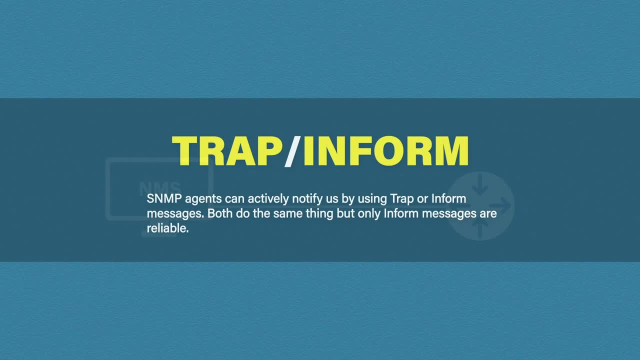 communicate back to the NMS. These are useful for monitoring critical events. The agent can send a TRAP or an INFORM to the NMS- the NMS- when an event occurs on the device, For example, if an interface goes down, the agent can. 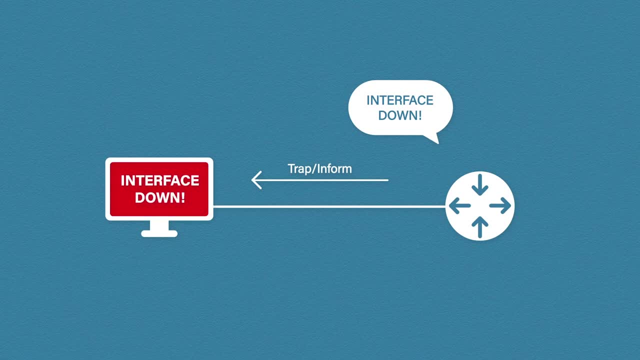 straight away, tell the NMS software with a trap or inform message. Traps and informs are two different types of messages, but they both do the same thing. The difference is that informs are reliable. An inform message will wait for an acknowledgement from the NMS. If it doesn't, 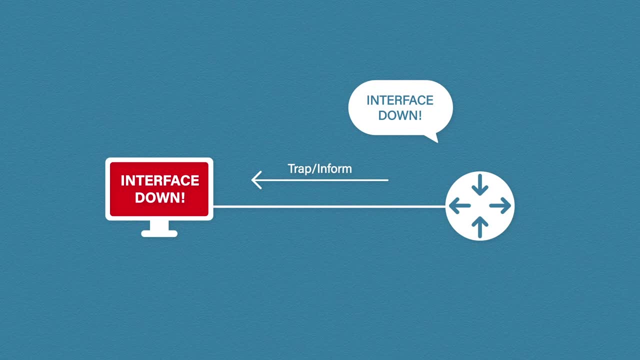 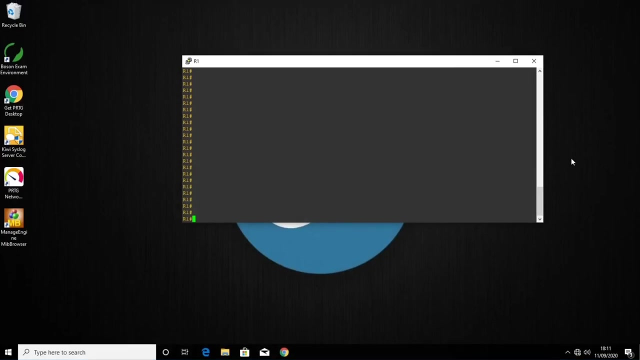 receive one, it will resend the inform. A trap, on the other hand, is sent and then forgotten. Even though informs are considered reliable, they both still use UDP. So now let's look at SNMP in action. Here is my PC which is acting as our NMS. I also have a connected router, which will be 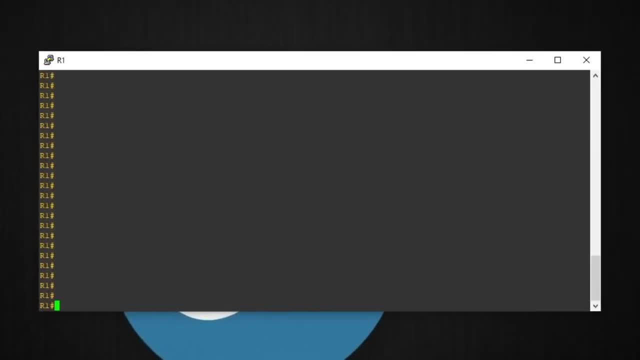 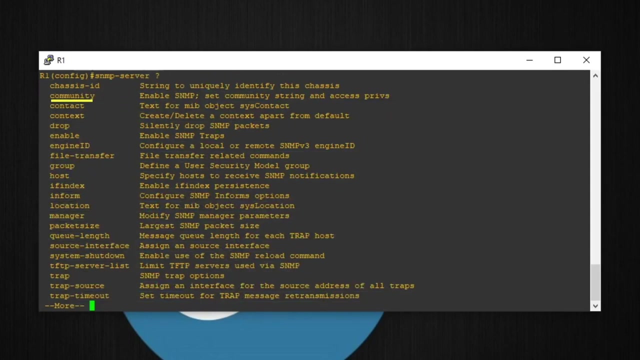 our SNMP agent. The first thing we need to do is configure the router to accept SNMP requests. So I'll go into global config by typing configure terminal. then I'll type SNMP server and we have several options here, but the one we want is community. The description says: 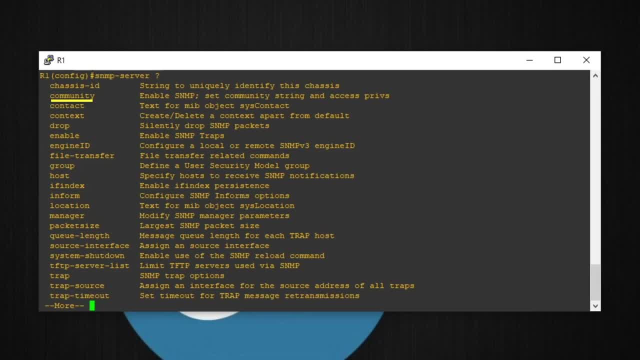 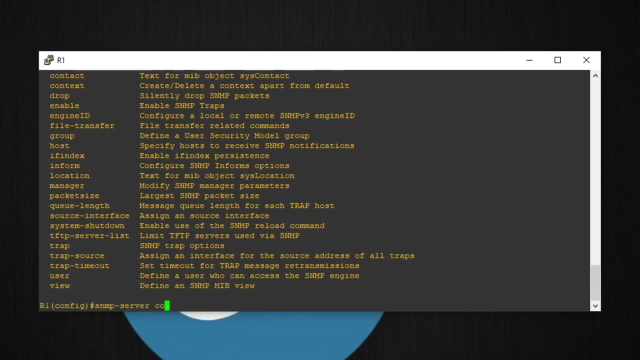 enable SNMP set the community string and access privilege. A community string is similar to a password. If a request is received with the correct community string, the agent will resist reply. So we need to type snmp-server- community and then we need to choose a text string In this. 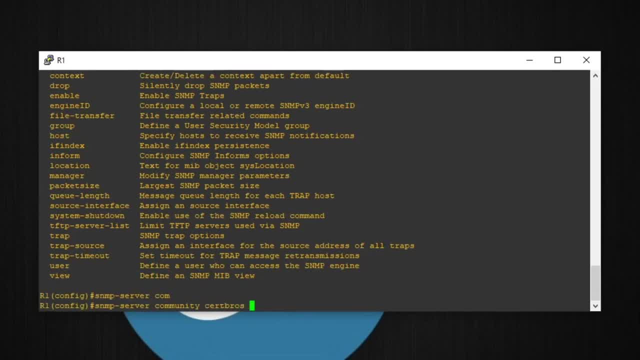 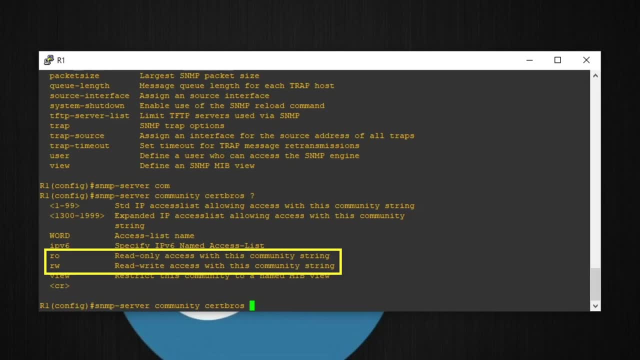 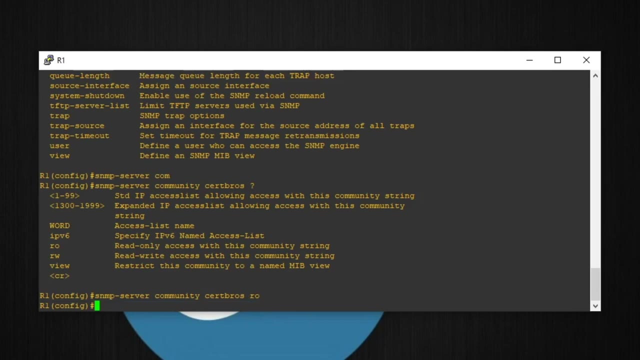 example, I'll just write search bros. If I then type question mark, you can see we have an option for read-only access and read-write access. I'll type ro for read-only access and press enter. but I also want write access, So I'll just press the up arrow on the keyboard. 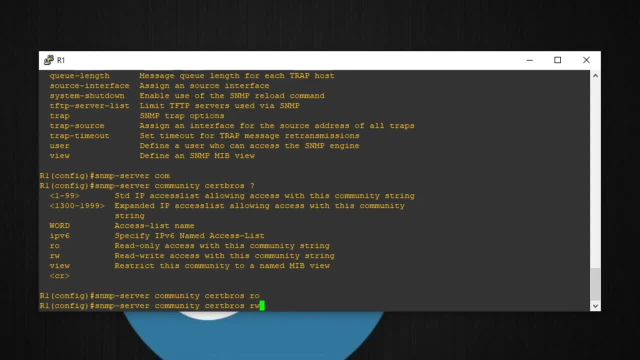 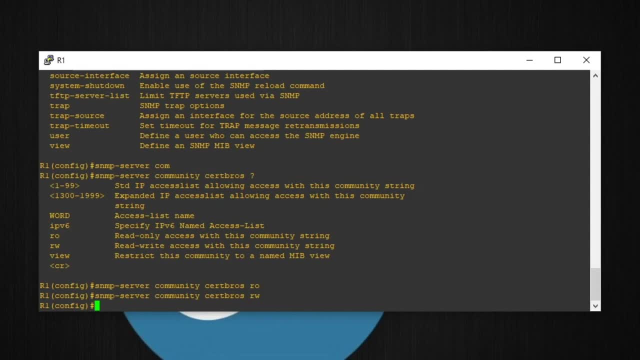 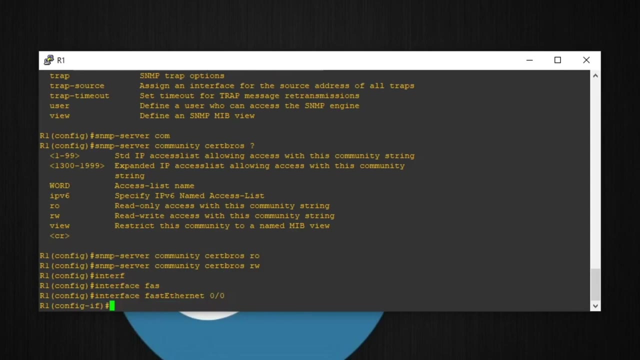 remove the ro and then type rw for write access. The last thing I need to do is configure an IP address on the router. I'll type interface fastethernet 0, slash 0, which is the interface connected to this computer. IP address: 192.168. 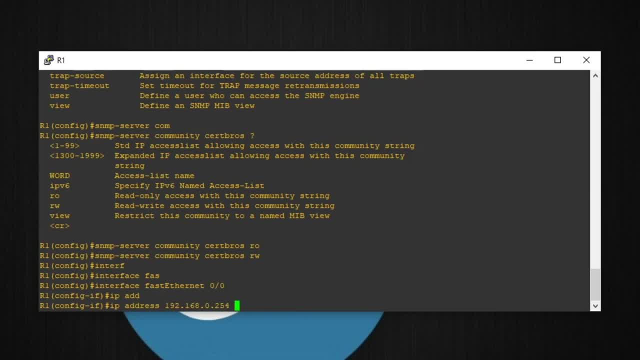 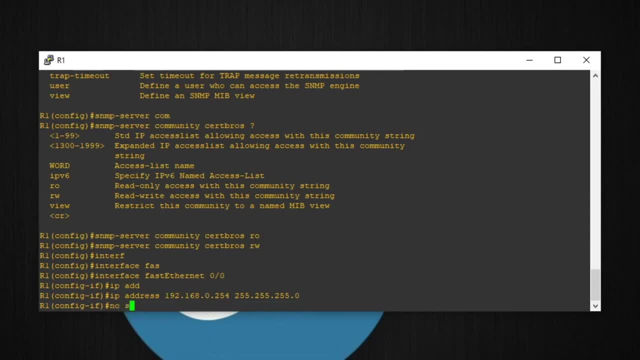 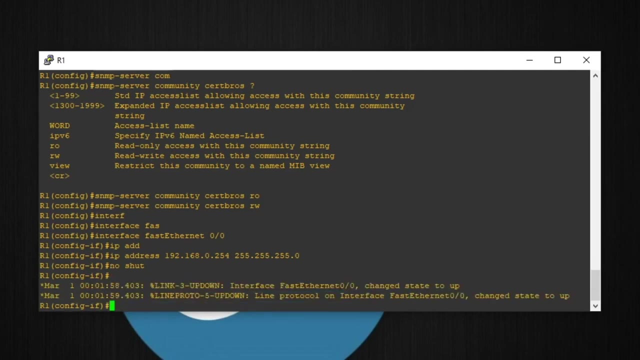 .0.254 with a subnet mask of 255.255.255.0, and then no shutdown to bring the interface up. With the interface now up, our router is ready to receive SNMP requests. So I'll minimize the router and I'm going to open this program called. 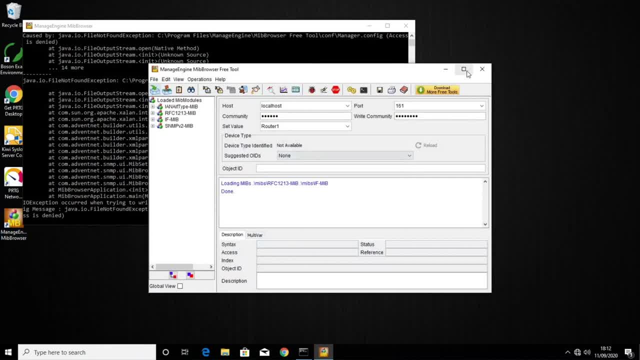 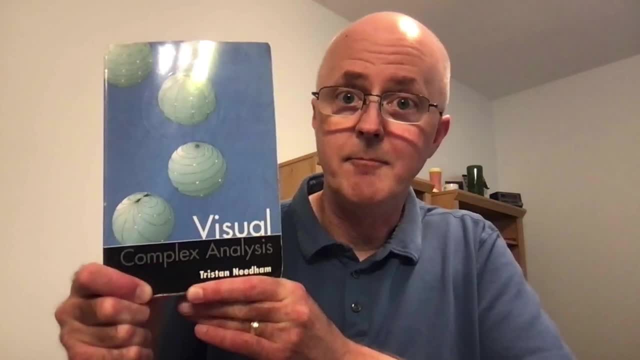 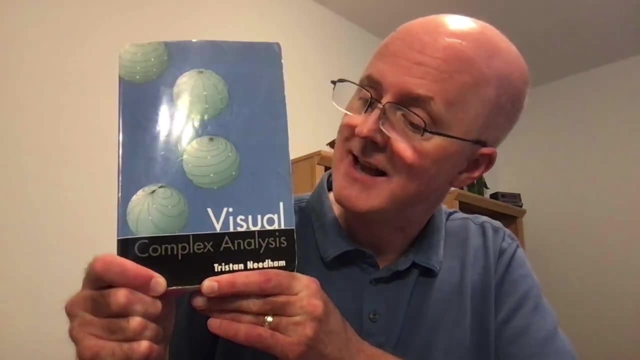 Complex numbers are beautiful, and the main purpose of this video is to illustrate that fact by looking at some of the pictures in this beautiful book called Visual Complex Analysis by Tristan Needham. I'll also show you some Mathematica demonstrations that illustrate the figures in chapter one of 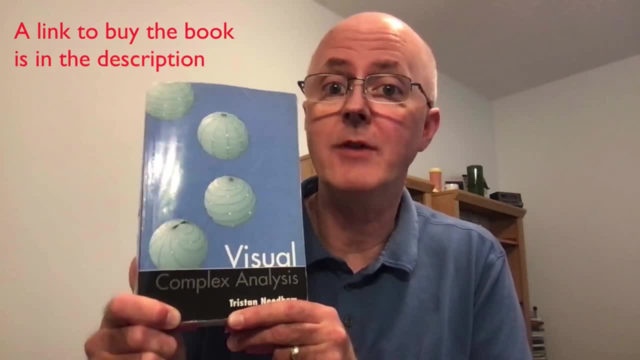 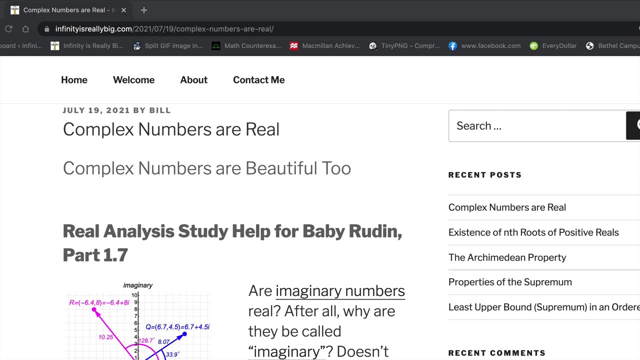 this book. I'll also make that Mathematica notebook available to anybody who wants to download it at a link in the description below. But before we get into looking at visual complex analysis, please indulge me for a few seconds while I mention that I posted an article at my blog: InfinityIsReallyBigcom. 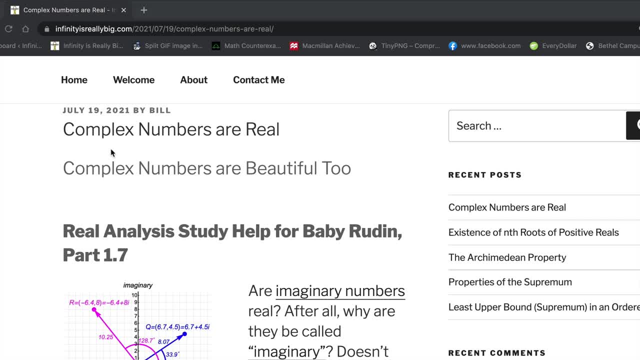 recently about complex numbers. I titled it: Complex Numbers Are Real, but a subtitle is that Complex Numbers Are Beautiful Too. It's part of my series on Real Analysis Study Help for Baby Rudin, a real analysis textbook that deals with complex numbers near the end of chapter one. So now let's get into looking at how.